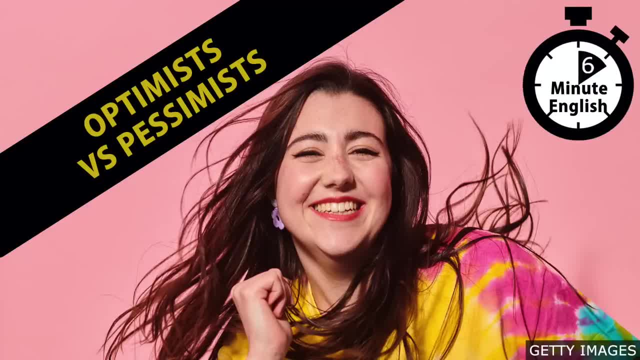 and that kind of tends to come across as being a bit of a Debbie Downer, when in actuality Germans just tend to be avid planners for all eventual negative eventualities as well. So that's kind of us being pessimistic but actually being cautious. 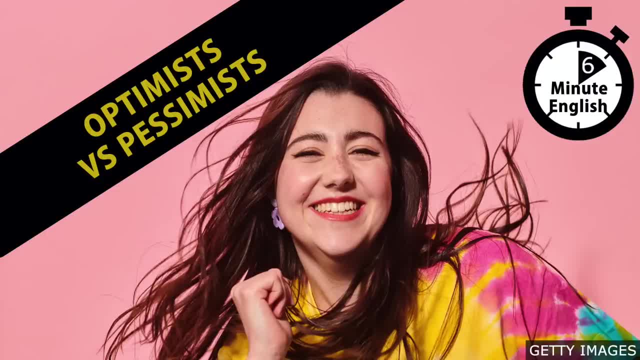 as opposed to, for example, what I've noticed in America, that a lot of people tend to be hyper-optimistic. I've always admired how Americans tend to be able… to sugarcoat everything. As a stereotypical pessimist, Hannah sometimes feels like a Debbie Downer. 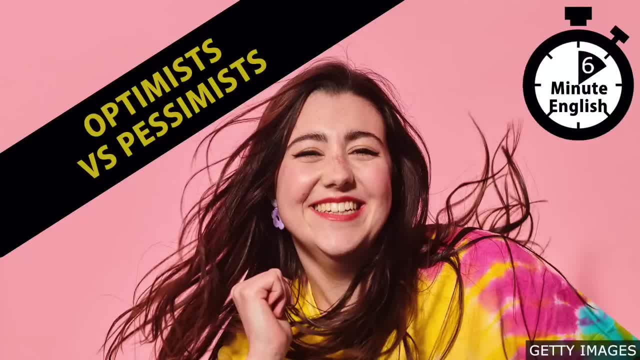 This expression is American slang for someone who makes others feel bad by focusing on the depressing aspects of things. Americans, on the other hand, are typically seen as optimists who tend to sugarcoat things, make things seem better than they really are. 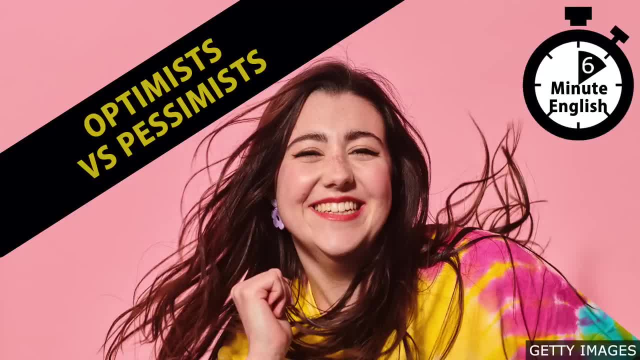 According to Hannah, many Americans are hyper-optimistic. She uses the prefix hyper- to say that there is too much of a certain quality. Hyper-sensitive people are too sensitive. A hyper-optimist is too optimistic. Besides, your country of birth age is another consideration in the optimism debate. 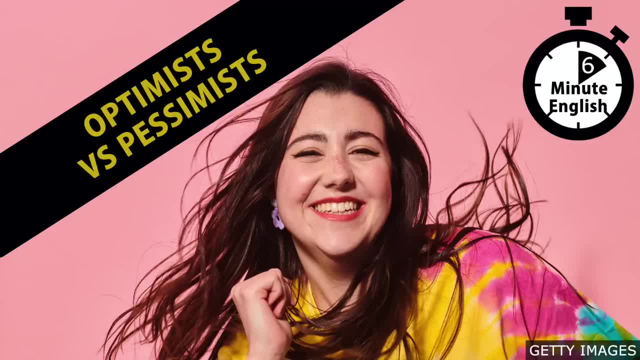 When we're young, we have our whole life ahead of us and it's easier to optimistically believe that everything's going to be all right. The belief that everything's going to be fine is called the optimism bias. It isn't fixed, but changes as we age. 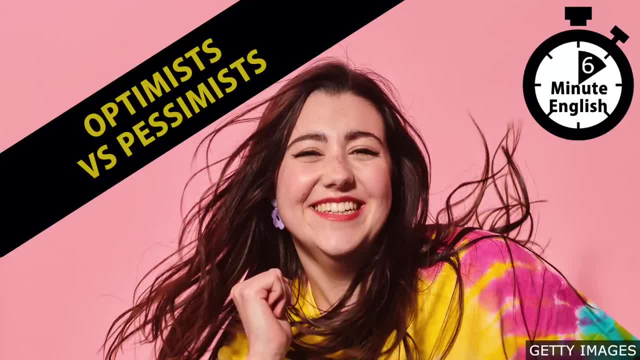 something neuroscientist Professor Tali Sherritt explained to BBC World Service programme CrowdScience. So it's quite high in kids and teenagers. They think, oh, everything's going to be fine, you know. And then it goes down, down, down and it hits rock bottom in your midlife. 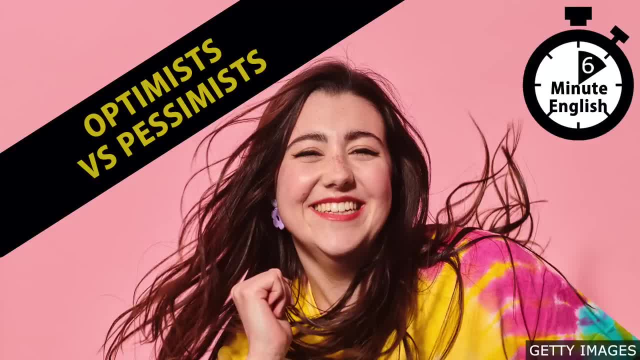 at which point the optimism bias is relatively small and then it starts climbing up again and it's quite high in the elderly population and that goes absolutely against our view of the grumpy old man or woman After starting out high in children. 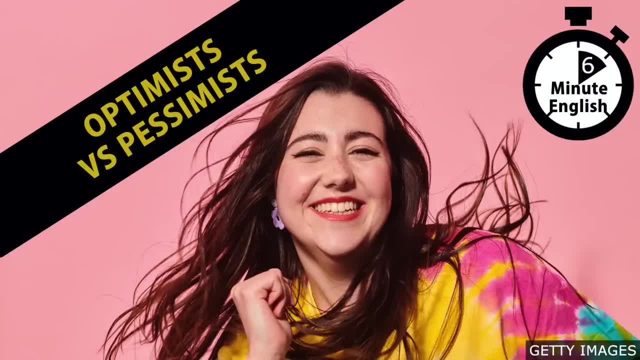 the optimism bias hits rock bottom, the lowest possible level in middle age, often because of work pressures, family responsibilities or caring for elderly parents. But optimism seems to increase again as we get older. This is surprising, as it goes against the image we have of the grumpy old man.